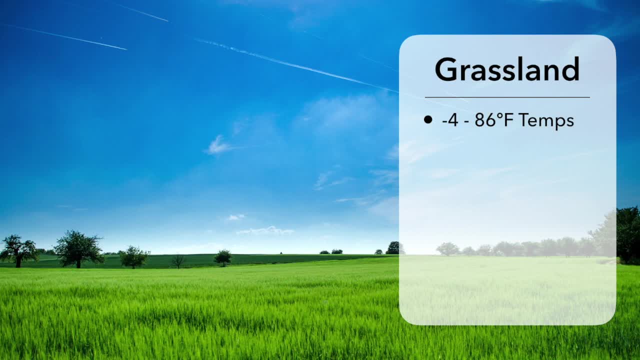 if you're in a grassland biome has to do with the temperature, which ranges from negative four to 86 degrees. on average, They have between 19 and 35 inches of annual precipitation or rainfall, And while you won't find many trees, there are many different types of grasses. 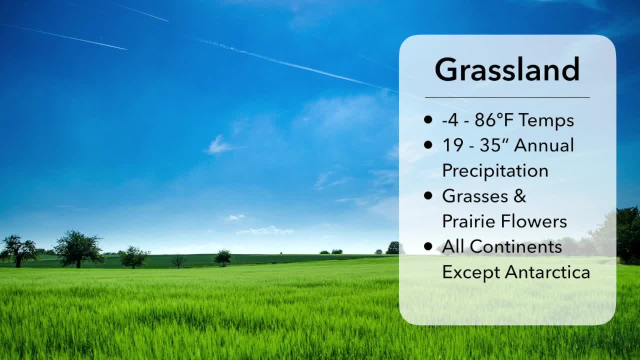 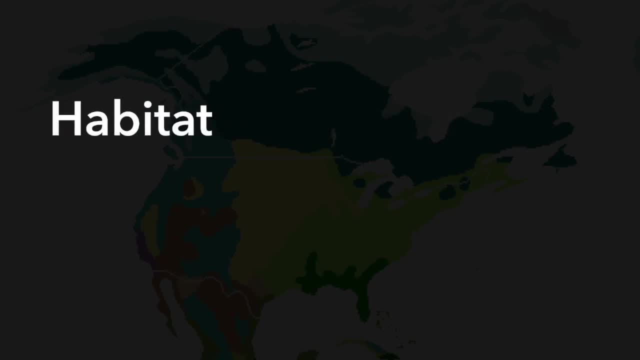 and prairie, flowers And grasslands can be found on every continent except Antarctica. Within those biomes are several different types of habitats, And a habitat is a place within a biome that supports the needs of an animal, And the basic needs for every animal is food, water and shelter. 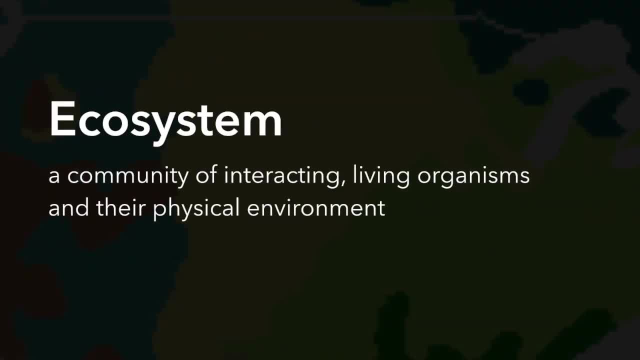 An ecosystem is a little bit different from a habitat, because the ecosystem looks at a community of interactive animals And the ecosystem looks at a community of interactive living organisms and their physical environment. So we're looking at the plants and the animals, but we're also looking at the physical environment around them, such as sun, lakes, rivers, oceans. 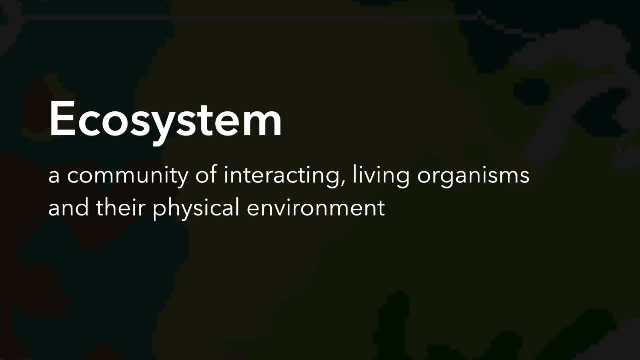 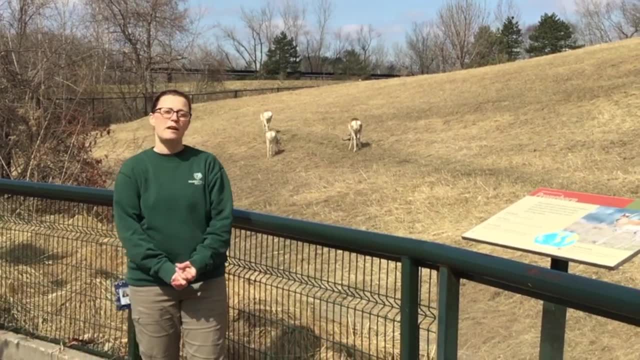 rocks anything else that's within their environment, even if it's not alive. Today we're in the grassland biome in a very important habitat, the Great Plains. This area runs right through the middle of the United States And it's a very important habitat for the 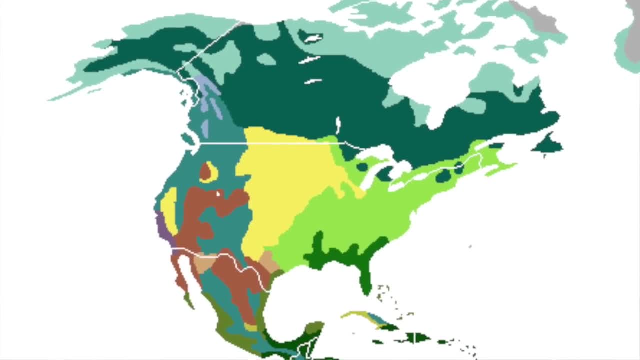 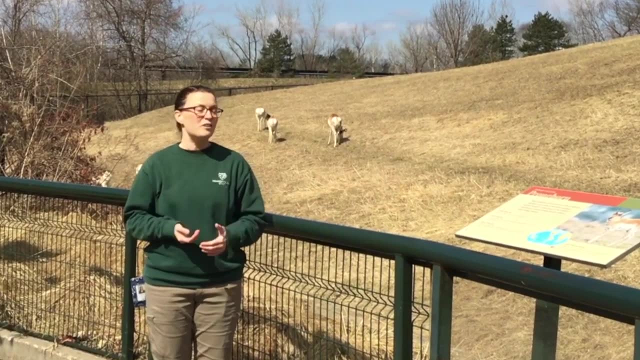 people of the United States in places like North Dakota, South Dakota and even Western Minnesota. It is known for its expansive prairies and fertile soil, And some of the animals you might meet here include pronghorns- seen here behind me- bison, prairie dogs, several. 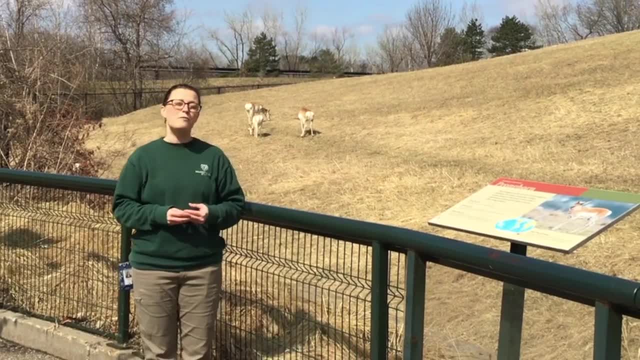 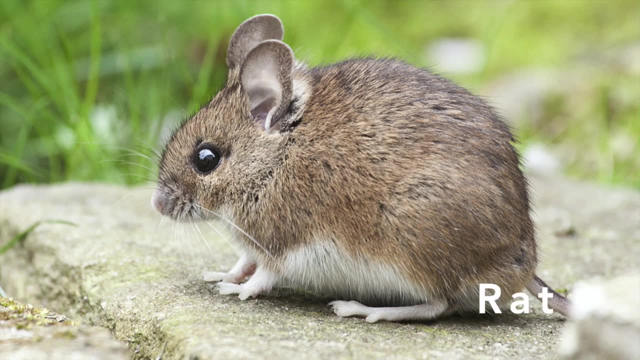 birds of prey and coyotes. We're gonna meet a few of these animals and learn more about how biomes, habitats and ecosystems are connected. Small rodents like mice and rats play an important role in many ecosystems And ст. 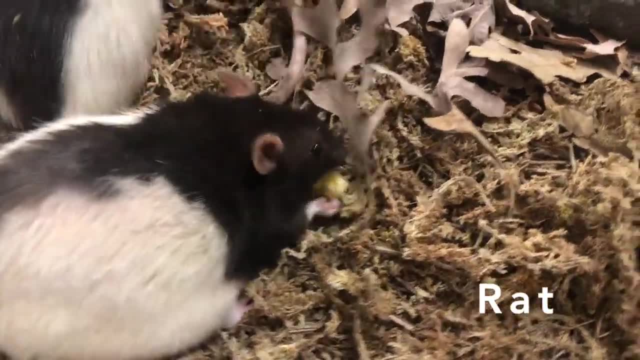 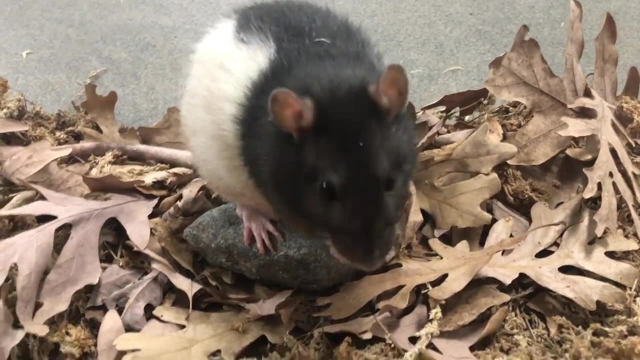 can be found on every continent except Antarctica. Rats are plentiful in the prairies of the Great Plains. Their job is a simple one: They are a main source of food for many types of animals found in this habitat. While their job may be, 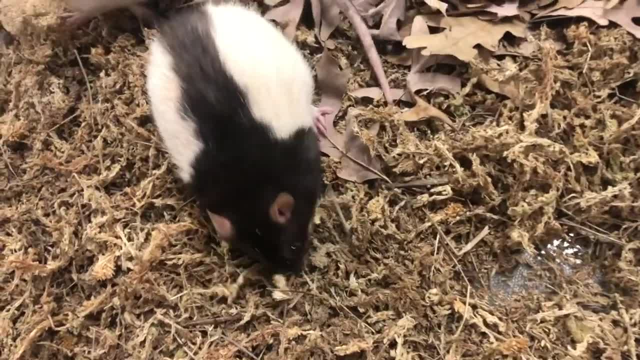 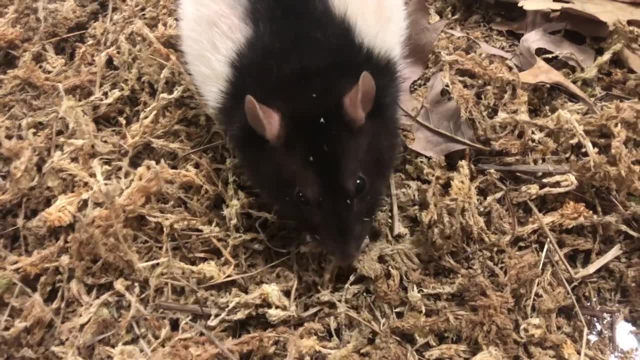 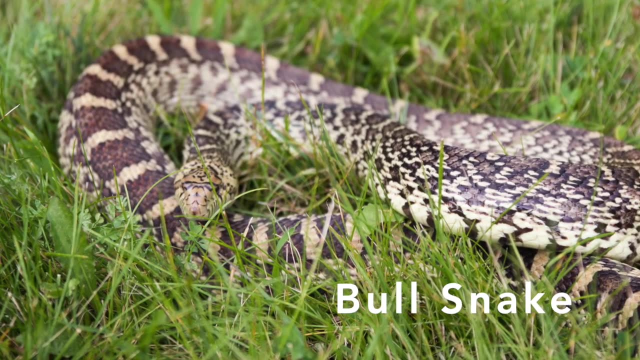 to allow other animals to eat. they are also very social and highly intelligent. Rodents have been known to outsmart the predators that chase them using well planned hiding places and intricate escape routes. Bull snakes are experts at utilizing the tall prairie grasses for camouflage and 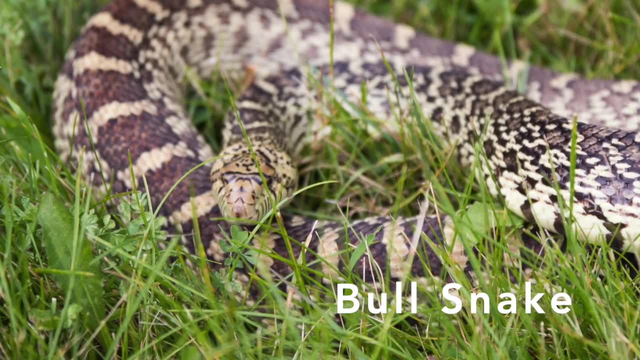 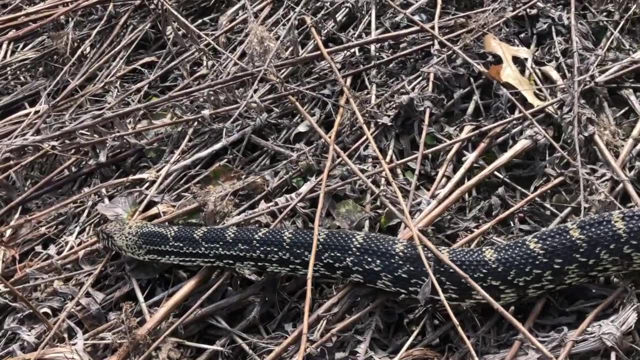 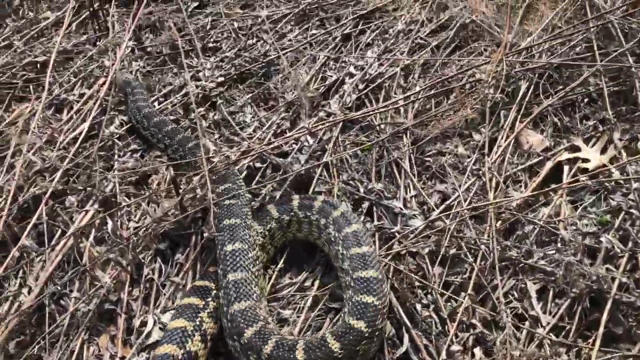 rely on rodents like rats for survival, as they make up much of the regular diet. These snakes are one of the largest found in Minnesota, growing up to six feet in length. Unlike rattlesnakes, who they are commonly mistaken for, this species is non-venomous and are very helpful to the farmers that share this. 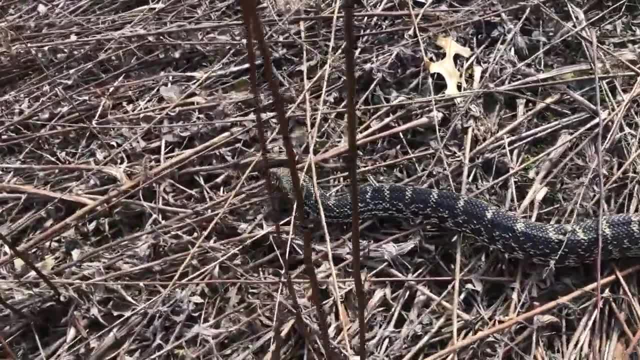 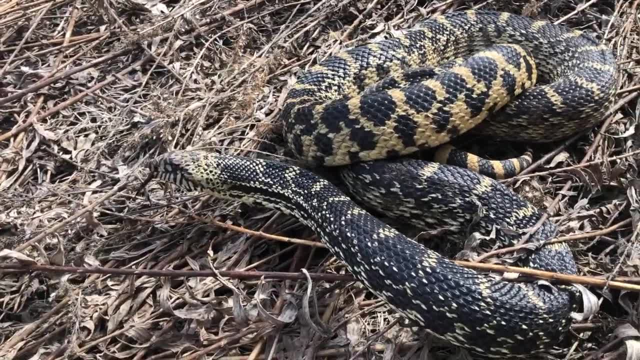 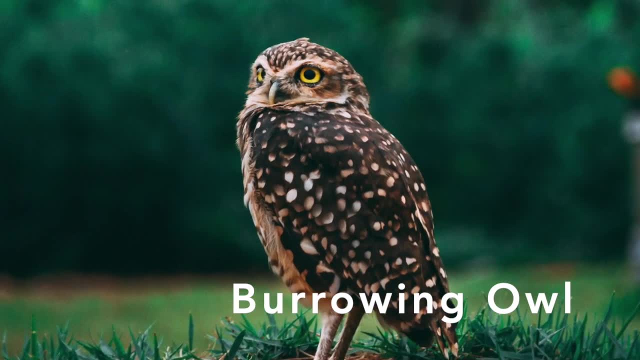 habitat. taking advantage of this habitat's fertile soil, Bull snakes help control the rodent population, Allowing more crops to be harvested. the rats, bull snakes and farmers all depend on each other. The next animal we're going to meet not only relies on mice, along with bugs, for food, but they also rely on another. 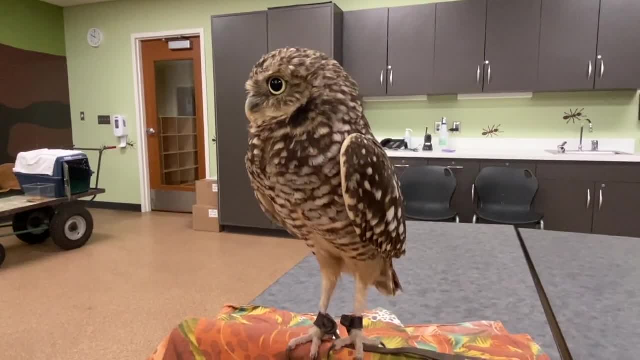 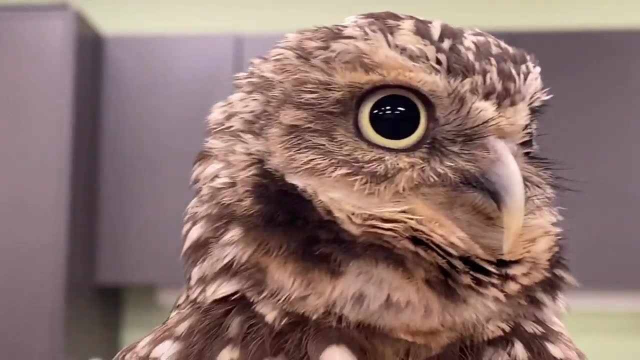 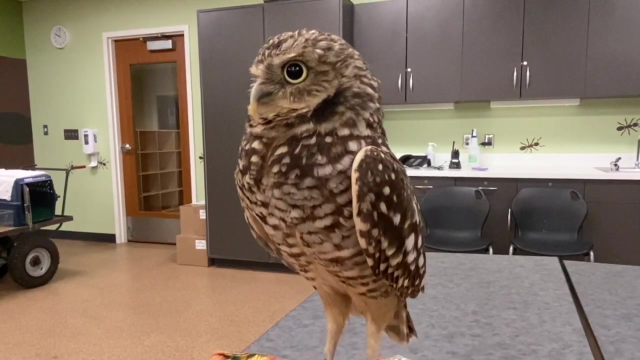 animal in their habitat to help supply them with shelter. This is a burrowing owl And while they are capable of digging their own burrow, these small owls depend on abandoned prairie dog towns to call home. Burrowing owls are solitary birds but live in communities out of convenience. These pre-made burrows create shelter. 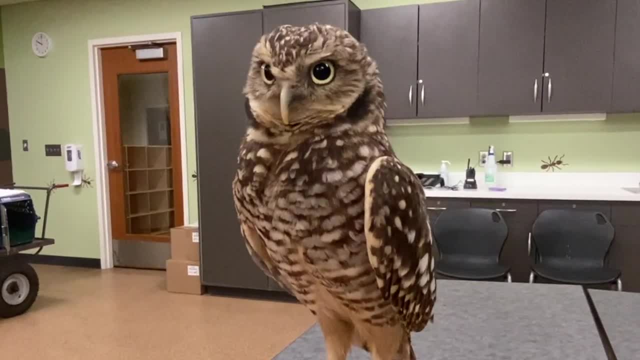 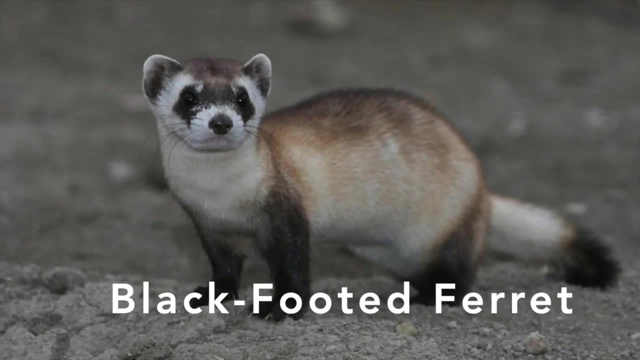 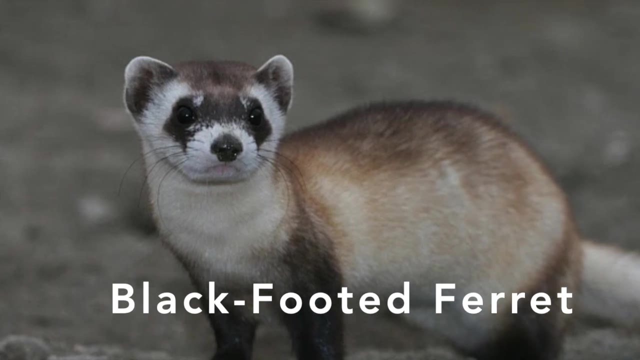 and safety, and living in large groups provide extra sets of eyes to watch out for predators like snakes and larger birds of prey. The history of black-footed ferrets are an amazing story about how ecosystems rely on all animals and their physical environment to survive. In the early 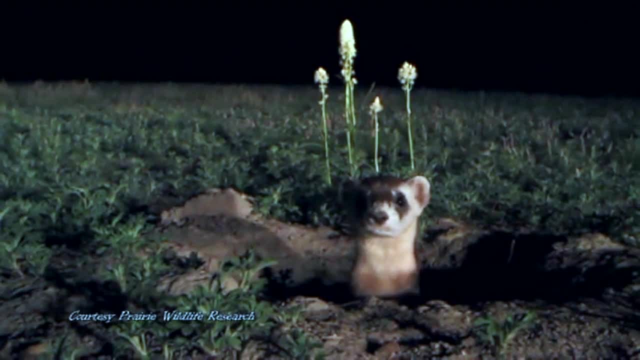 1900s, agriculture was booming in the Great Plains. One big problem farmers and ranchers were having involved the expanse of prairie dog towns that impacted their ability to expand their farmland. To solve their problem, farmers and ranchers, along with the local government, exterminated. 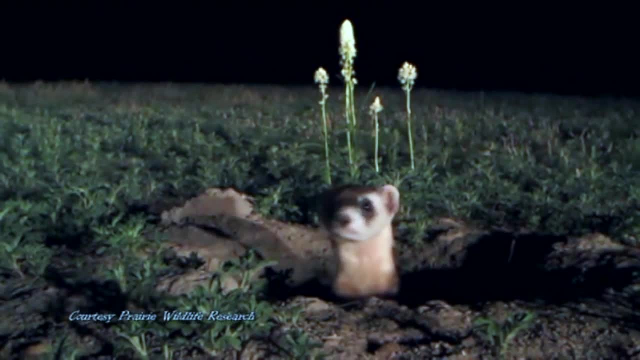 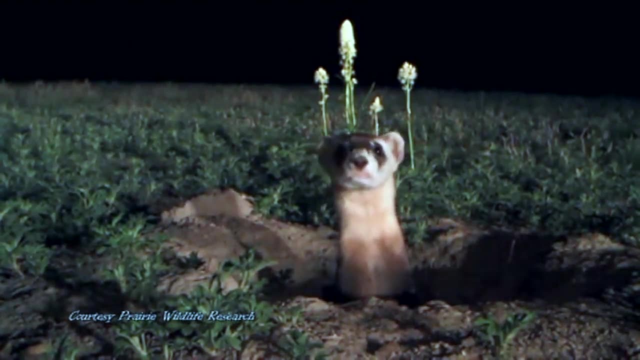 prairie dogs from the ecosystem. The black-footed ferret, whose diet relies on prairie dogs for survival, lost their food source and were declared extinct in 1979.. Several years later, 18 wild individual ferrets were captured and a breeding program was initiated to bring back and reintroduce.